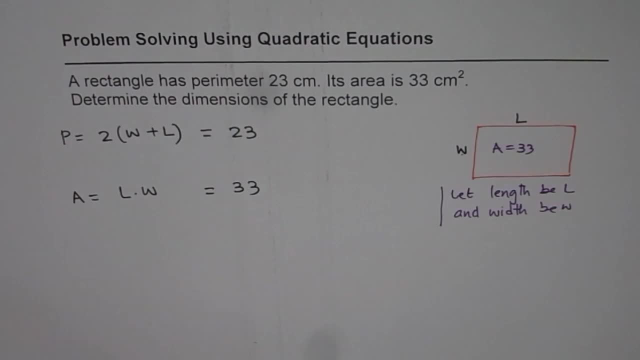 here, area equals to 33.. That kind of helps you to understand the question better. Now the situation is that we have two different equations and two variables. So whenever that is the situation, we have to write one variable in terms of the other. Now, in this particular, 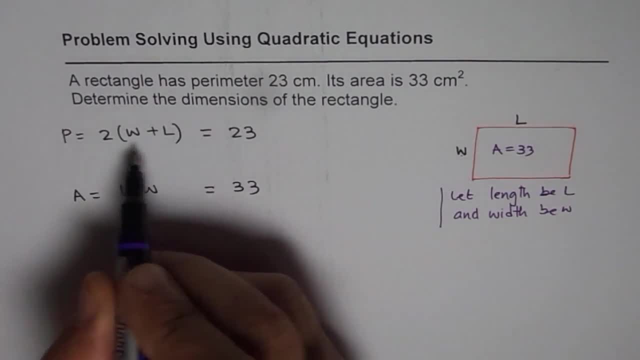 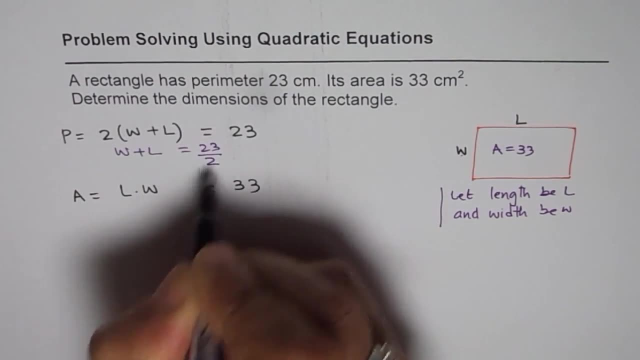 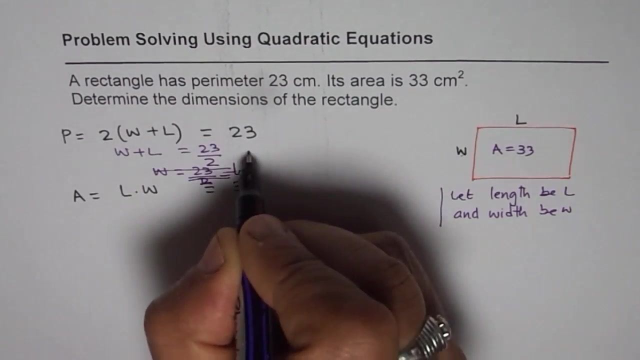 case fractions are involved. So what we will do is we will say: well, we can say: w plus 1 is equals to 23 divided by 2. or we can say: width is equals to 23 divided by 2 minus l. Sorry, I have to write 2 here, So let me rewrite this. So width is equals to. let me. 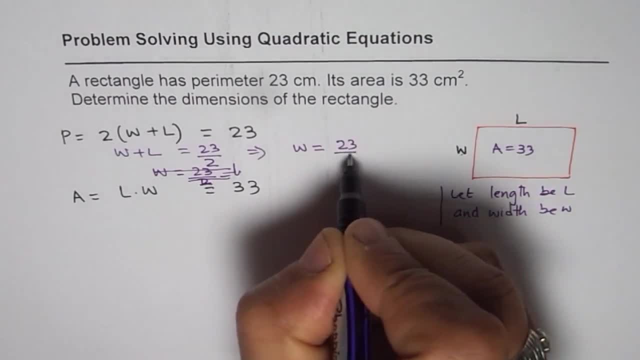 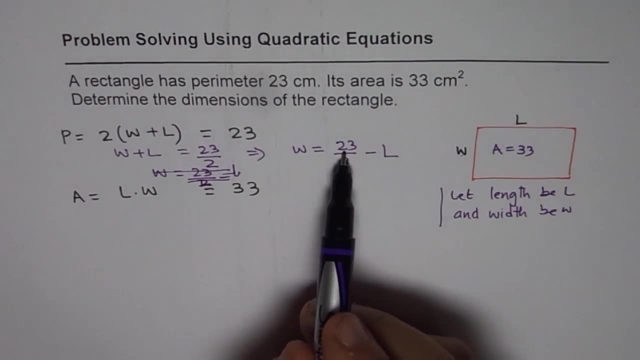 write here: Width is equals to 23 divided by 2 minus l, So we get one variable. in terms of the other variable, This can be substituted in the same second equation, so you'll have equation in one variable only, right? so instead of width w, i will 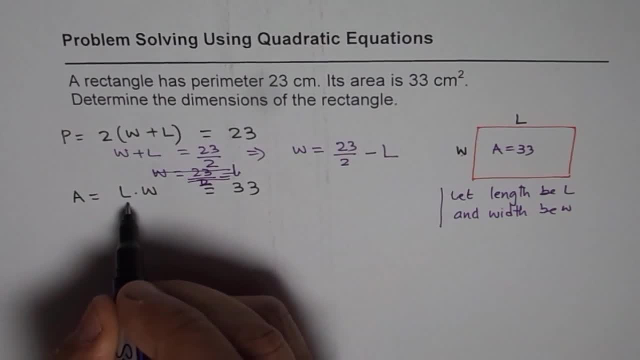 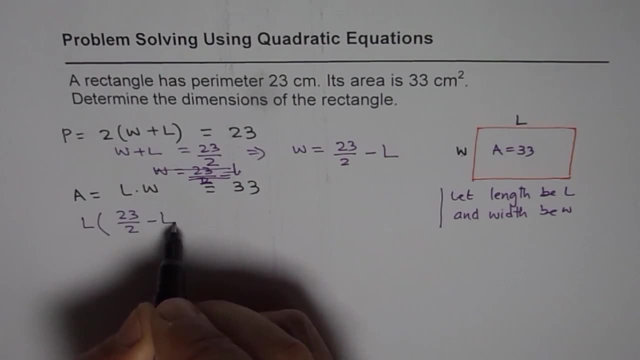 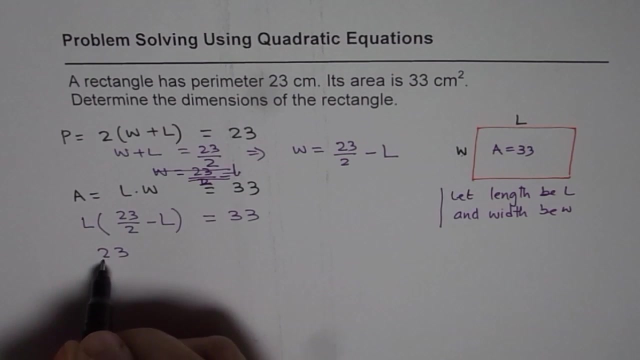 write 23 divided by 2 minus l. so instead of width, i'm writing, so i'll get l times. 23 divided by 2 minus l equals to 33. now if you open this bracket, you get 23 divided by 2 l minus l square. 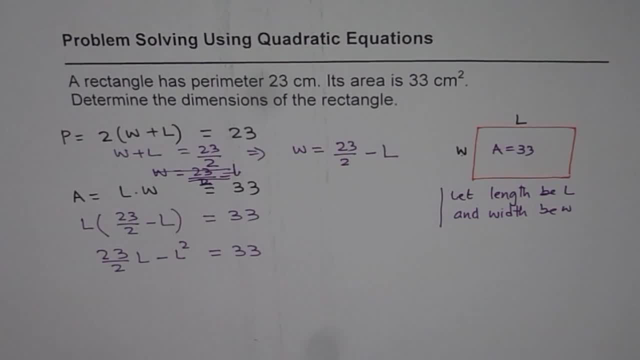 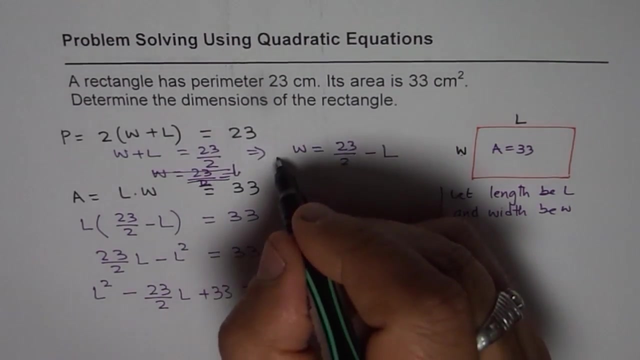 equals to 33, correct? so you get a quadratic equation which you can rearrange and you can write l square bringing all these terms to the right: minus 23 divided by 2, l plus 33 equals to 0, right? so some of you might be feeling uncomfortable with this fraction, which i'm 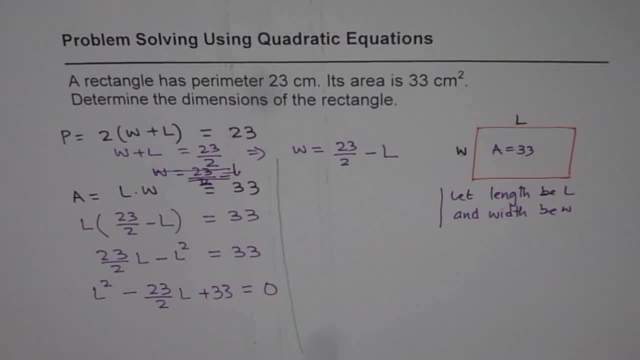 carrying forward for such a long time. well, at times you can also write this as as a decimal value, right, and then at this stage we can actually use quadratic formula and find the value of l right. so let me write this equation with decimal values and then we will use quadratic formula, so we could write this as l squared. 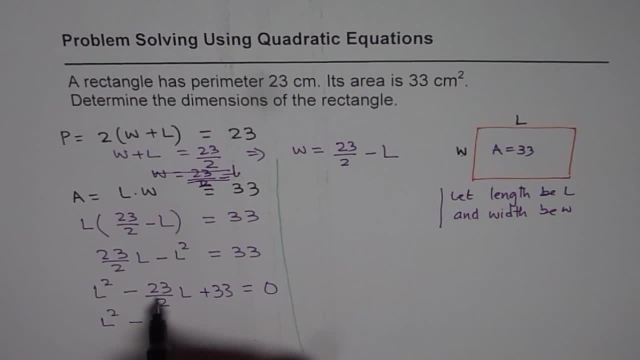 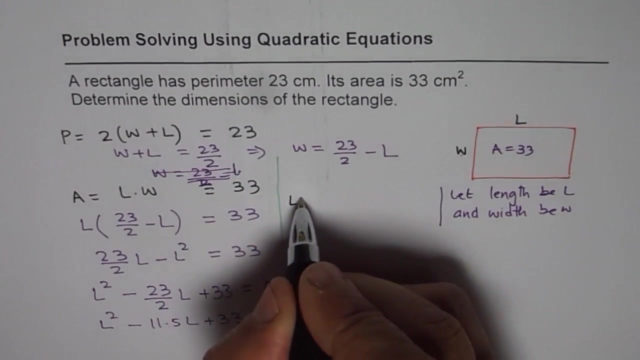 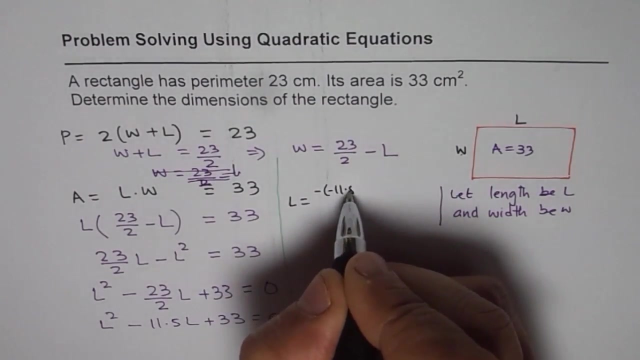 minus 23, half of 23, half of 22 is 11, so it gives 11.5. l plus 33 equals to 0, right? so that's it. right now we will use quadratic formula to find the value of l. quadratic formula is: l equals to minus of b value, which is minus of minus 11.5. let me write like: 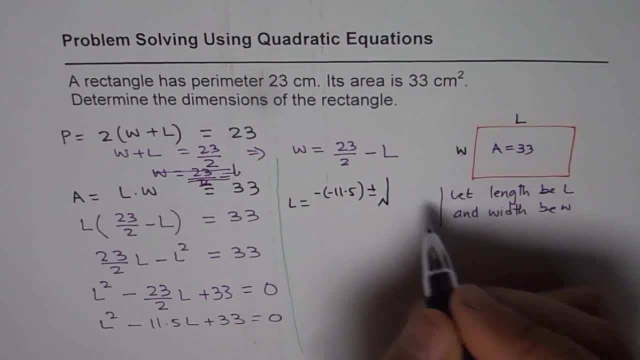 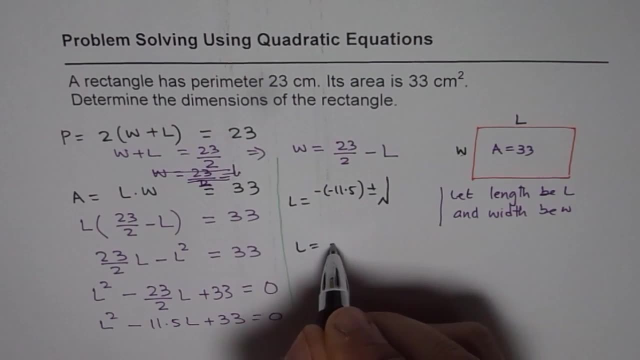 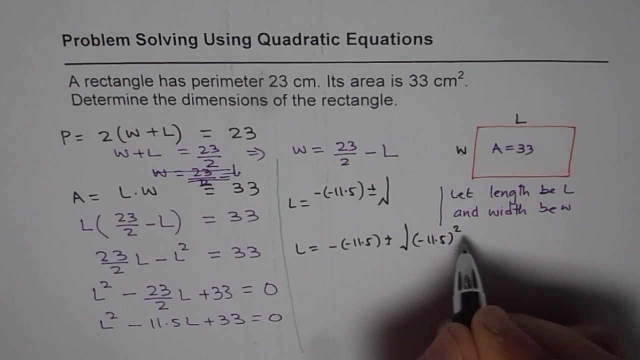 this plus or minus square root of this square. okay, so we'll run out of space here. okay, so let me rewrite this here: l equals to minus of minus 11.5 plus minus square root of minus 11.5. whole square minus 4 times a, which is 1, and c is 33 square root divided by 2 at this stage. 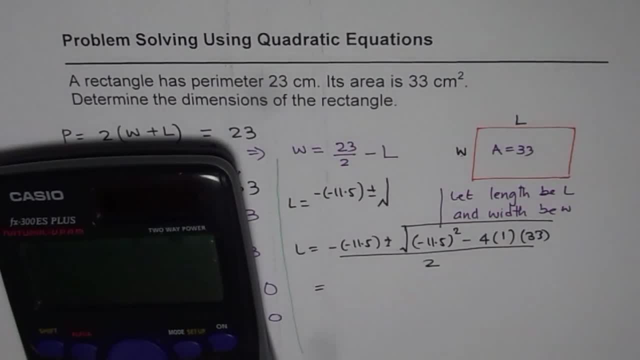 you have to take help of calculator. so take the help of the calculator, figure out what is there within the square root. so square root: 11.5, square. no need to write minus, since square of minus is plus correct. minus 4 times 33, 4 times 33 equals to that- gives you half, which in decimals will be 0.5. 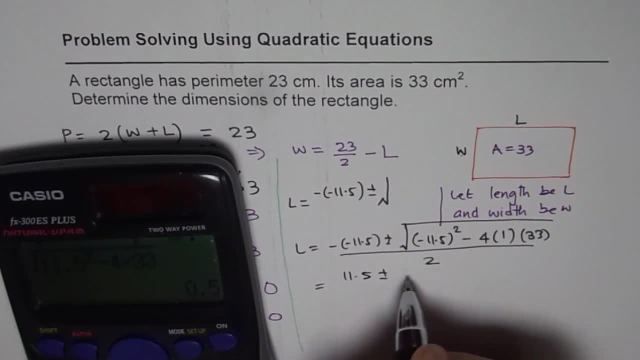 so what we get here is 11.5 plus minus 0.5 divided by 2. right, so we get two values. you can use any one of them first. then let's use 0.5 plus first, then we get 11.5, that is 12. 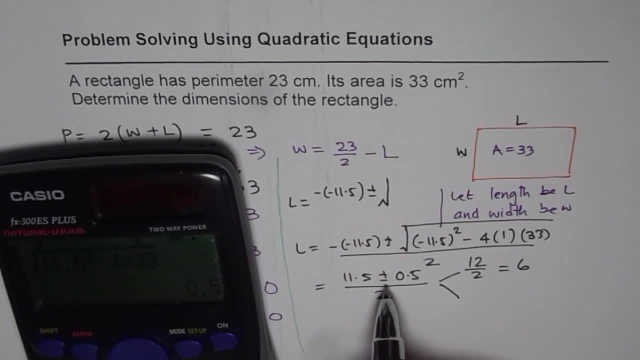 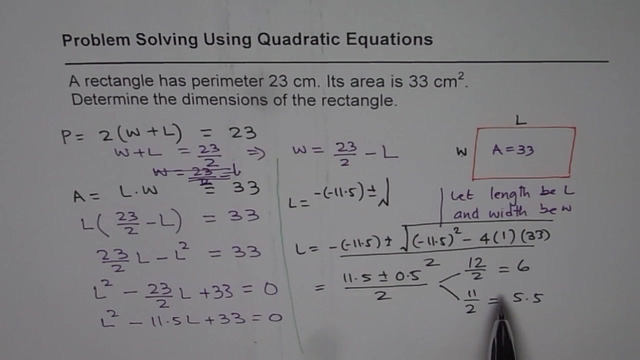 divided by 2 will give us 6. if i use the negative value, then i get 11 divided by 2, which is 5.5. so these are two possible values of the length l. now, once we know this length l, then we can find. 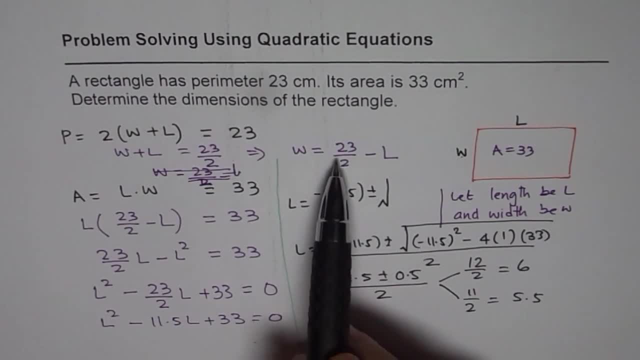 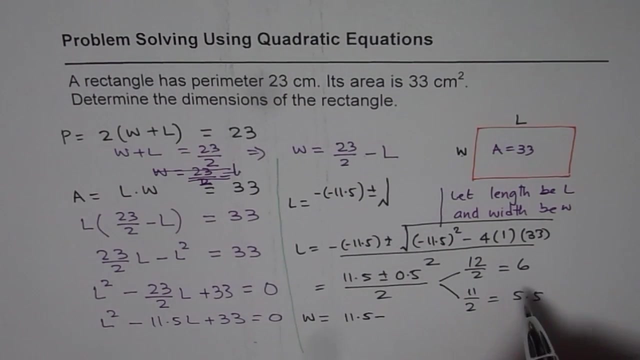 width right. so width is, as you can see from here, 11.5 minus l, correct, so width will be 11.5. i could write this as 11.5 minus l, so 11.5 minus. choose any one of them. so if i choose 6 for,